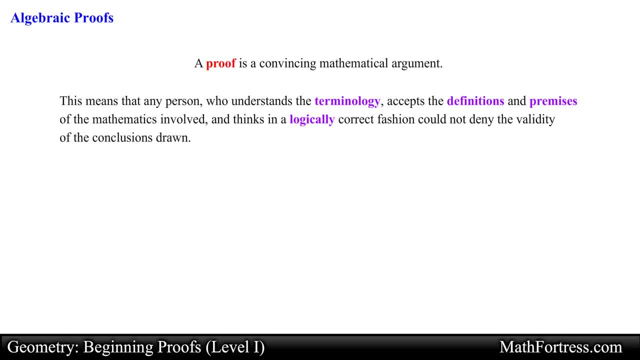 premises of the mathematics involved and thinks in a logically correct fashion, could not deny what that firm meaning, why the validity of the conclusion is drawn When describing the solution of an equation as an algebraic proof. the premises for the proof are the given equation, the properties of equality and the properties of real numbers. 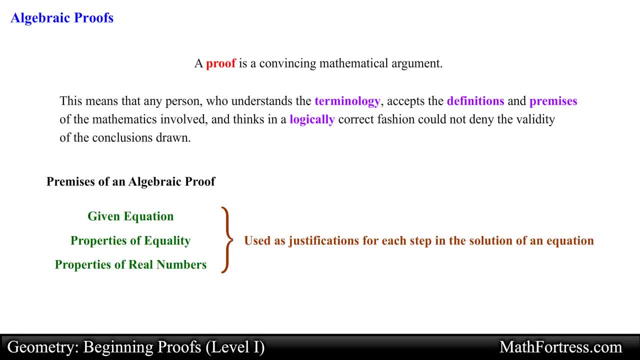 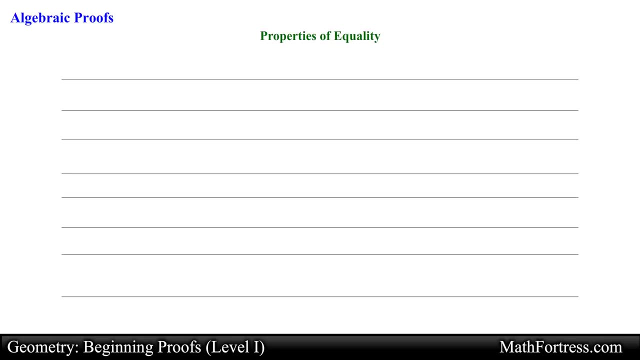 These premises may be used as justifications for each step in the solution of an equation. The process is analogous to the process used when writing geometric proofs. An algebraic proof uses algebraic properties of equality. Recall from your beginning algebra course that the properties of equality include the: 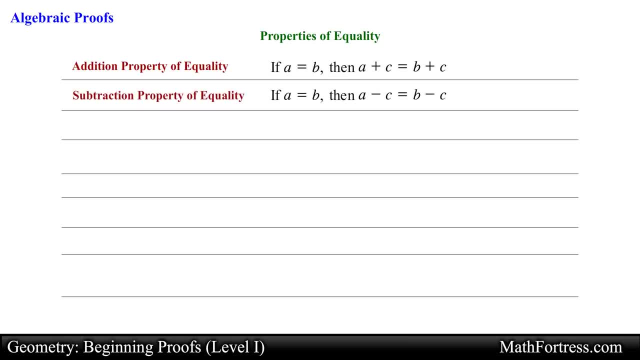 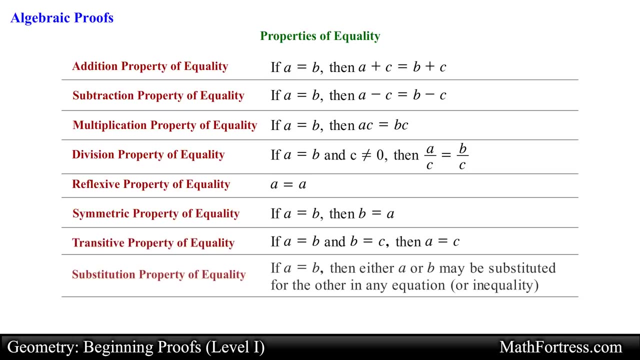 addition, property of equality, subtraction, property of equality, multiplication, property of equality, division, property of equality, reflexive property of equality, symmetric property of equality, transitive property of equality and substitution property of equality. An algebraic proof also uses the distributive property. 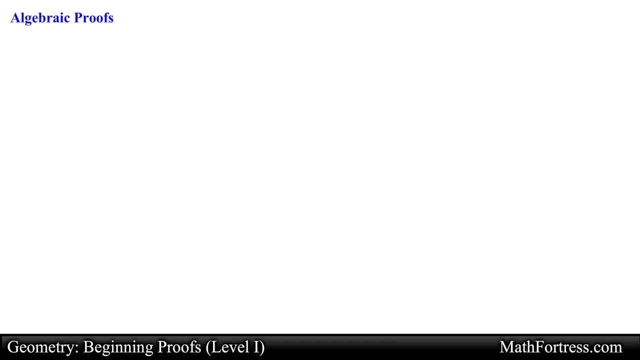 An important part of writing a proof involves the justification of every step. For example, say that we want to solve the following equation and we are asked to prove it. We start our two column proof by writing the equation on the left column as follows: We will write all of our statements on the left column, creating a new line for each statement. 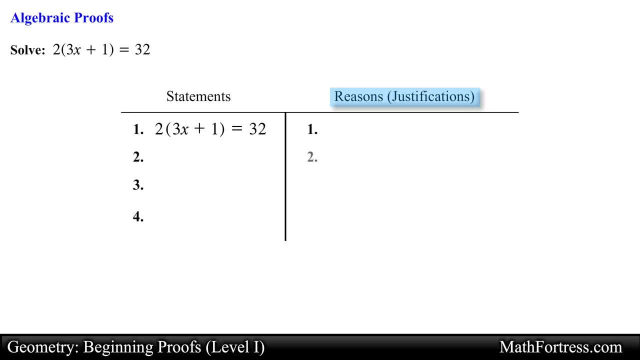 On the right column we will write out our reasons or justifications of the statements from the left column. Each statement must be numbered and correspond to a reason which has the same number as a statement in the left column. Each numbered statement and reason must originate on the same line. 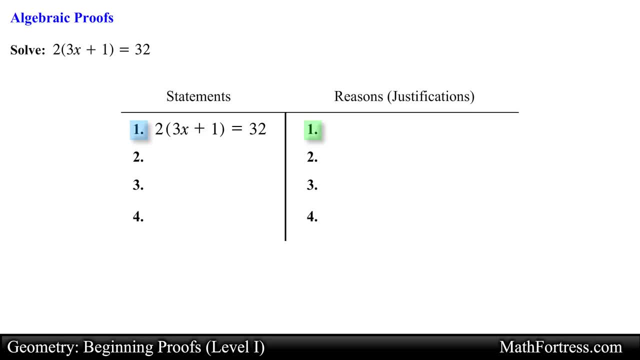 Usually the first statements in a proof will be given to you. In this case we are given this equation, so the justification or reason for this statement will be given equation. Next we proceed in solving the equation. So we first apply the distributive property and distribute 2 into each term. 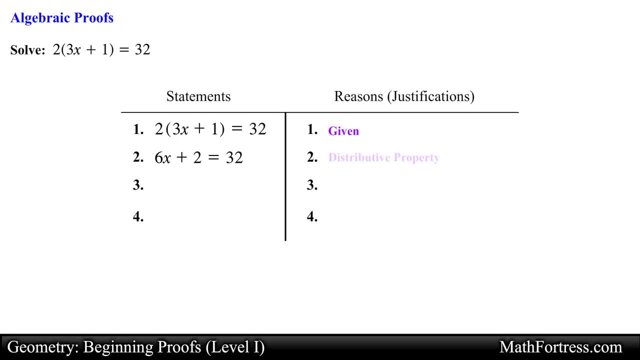 We then write the reason or justification for this step. In this case, we write distributive property, since we applied the distributive property to obtain the new statement. Next we subtract 2 from both sides of the equation and simplify. Now this is where many students make a very common mistake. 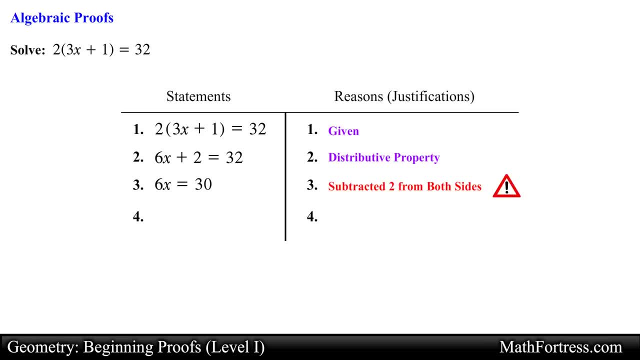 Many students would write subtracted 2 from both sides as a reason or justification. This would be an incorrect reason. The correct reason needs to make use of the properties of equality. In this case, we use the subtraction property of equality. The justification for each step is not simply a description of the operation, but rather 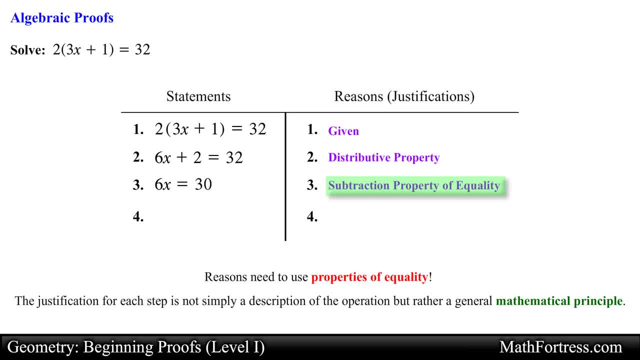 a general mathematical principle. So make sure you use a mathematical principle as a justification. The last step is to divide both sides of the equation by 6.. Doing that, we obtain x equals 5.. For our justification we write division, property of equality, and not divide by 6.. 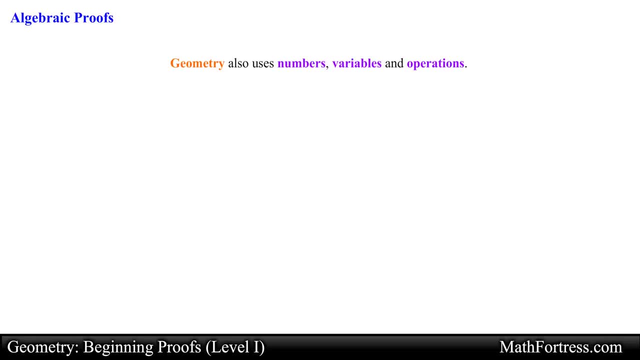 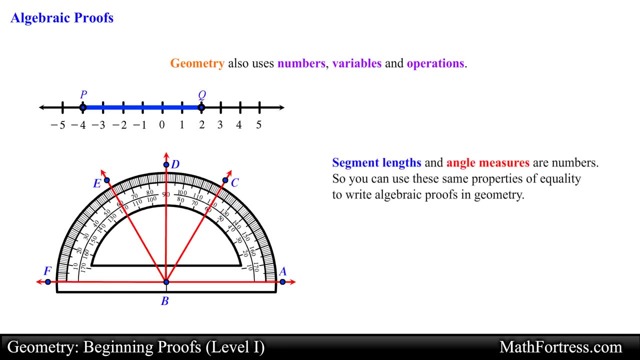 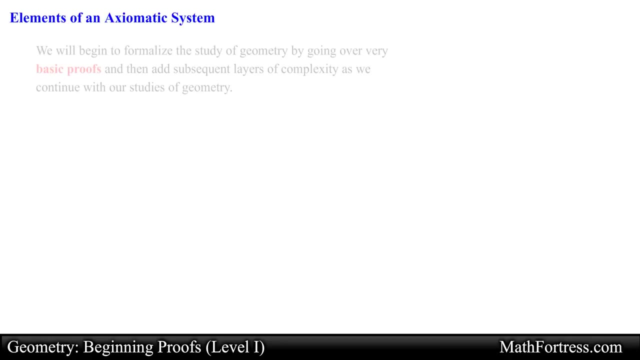 Like algebra, geometry also uses numbers, variables and operations. For example, segment lengths and angle measures are numbers, So you can use these same properties of equality to write algebraic proofs in geometry. We will begin to formalize the study of geometry by going over very basic proofs and then add: 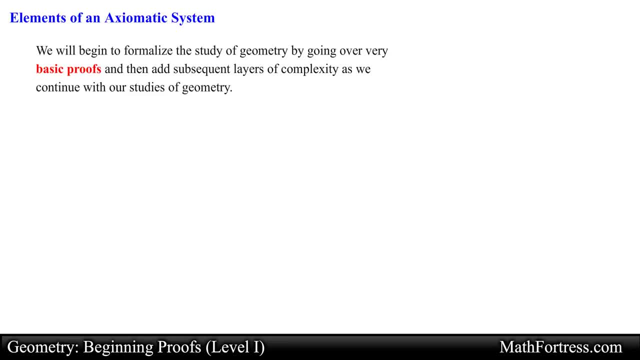 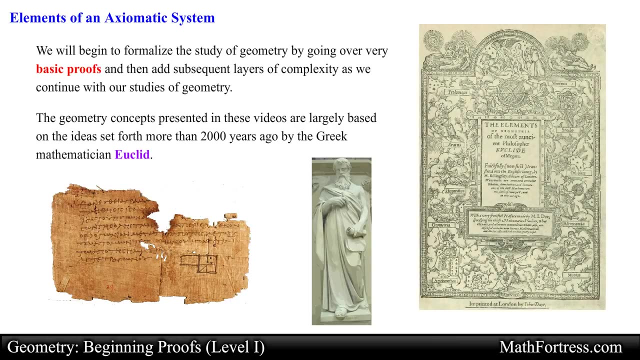 subsequent layers of complexity as we continue with our studies of geometry. The geometry concepts presented in these videos are largely based on the ideas set forth more than 2000 years ago by the Greek mathematician Euclid. His series of books Elements is the first known work in 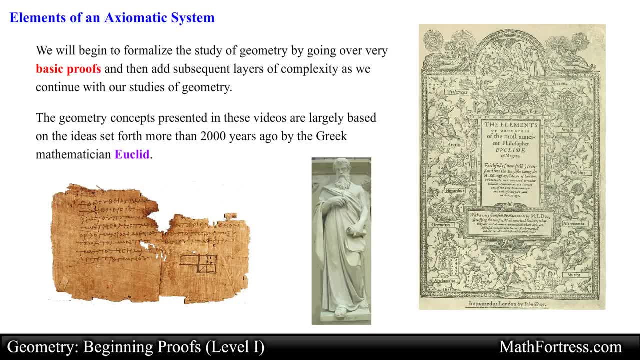 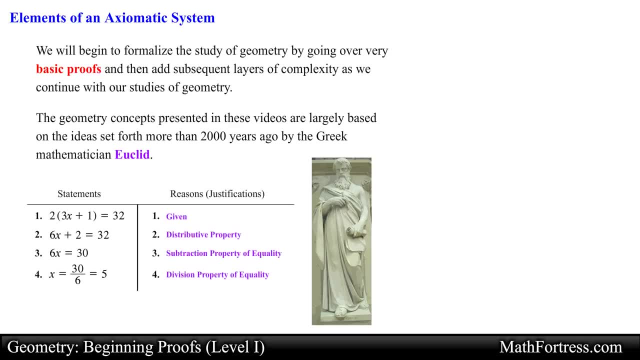 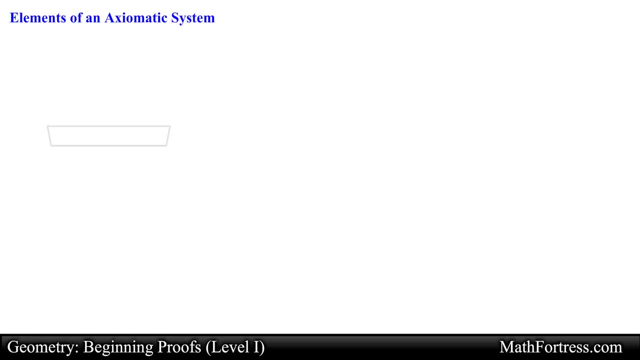 which a logical deductive system of reasoning is used as a means of unifying all mathematical knowledge. In that spirit, geometric proofs will help us learn how to build a logically coherent system of facts by using deductive reasoning. Geometry is based on an axiomatic system. 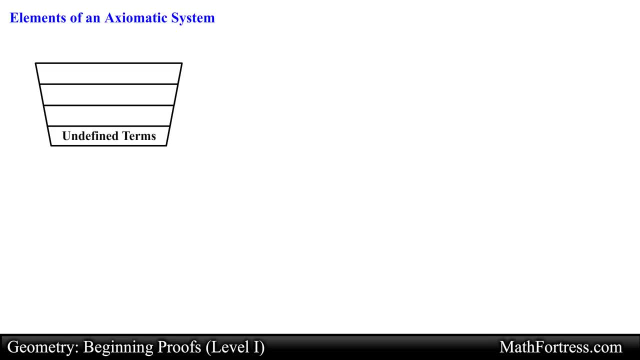 A modern axiomatic system begins with a small set of undefined terms and builds through the addition of definitions and postulates to the point where the axiomatic system is defined, Where many rich mathematical theorems can be proved In an axiomatic system. we agree to leave some terms undefined and then build definitions. 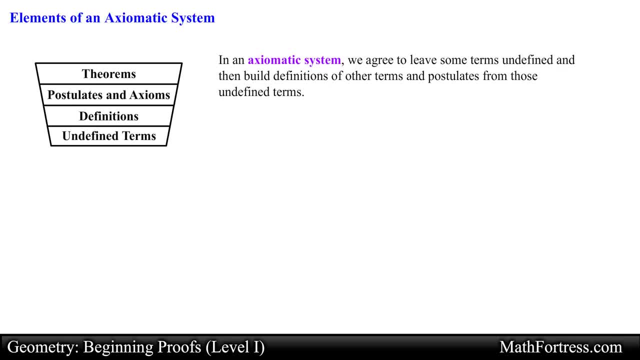 of other terms and postulates from those undefined terms. Undefined terms can be described, but cannot be given precise definitions using simple known terms. Three undefined terms in geometry are point, line and plane. Recall that a point is a circular dot That is shrunk until it has no size. 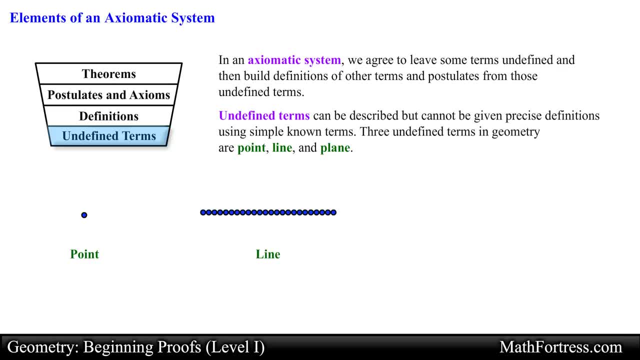 A line is formed by an infinite number of points, It also has an infinite length, so we denote this idea by using arrowheads. Also, a line has no thickness. A plane is a sheet of paper formed by an infinite number of points, with no thickness and extending. 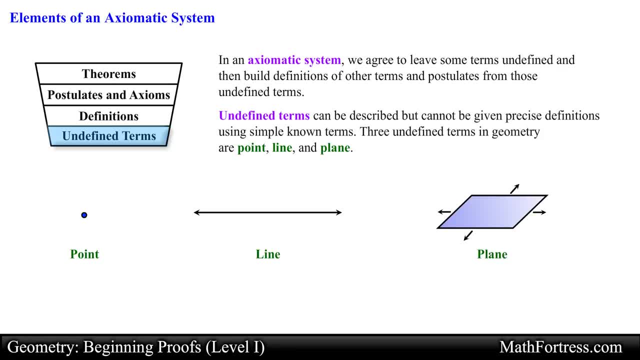 infinitely in all directions. Although a plane has no edges, we usually picture a plane by drawing a four sided figure. We often label a plane with a capital letter. These descriptions provide a way for us to visualize points, lines and planes, but they are not definitions. 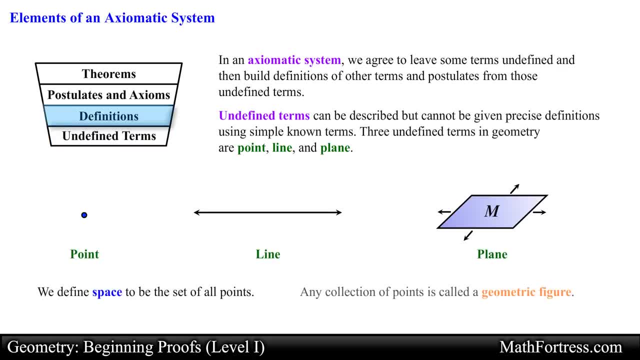 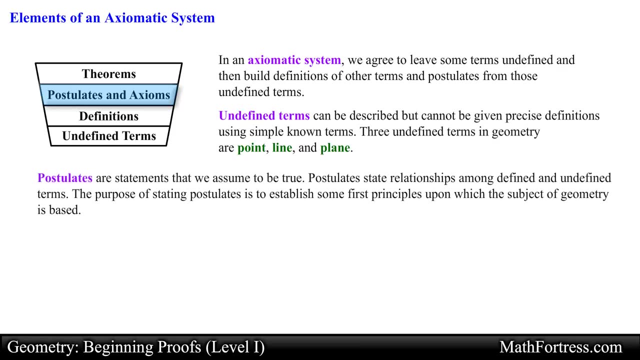 We define space to be the set of all points. Any collection of points is called a geometric figure. In particular, lines and planes are composed of points and hence are geometric figures, Postulates or statements. Postulates are statements that we assume to be true. 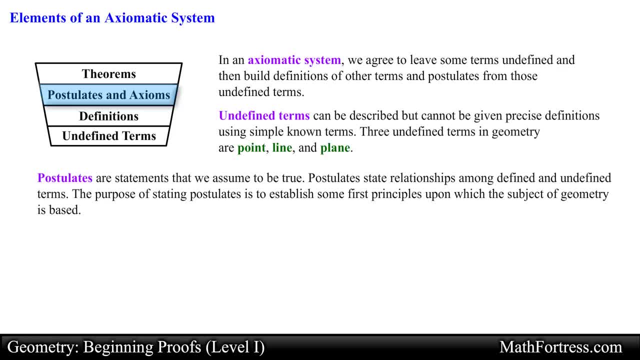 Postulates state relationships among defined and undefined terms. The purpose of stating postulates is to establish some first principles upon which the subject of geometry is based. After introducing postulates and some definitions, we may deduce new results, Results that we deduce from undefined terms, definitions, postulates or results that follow. 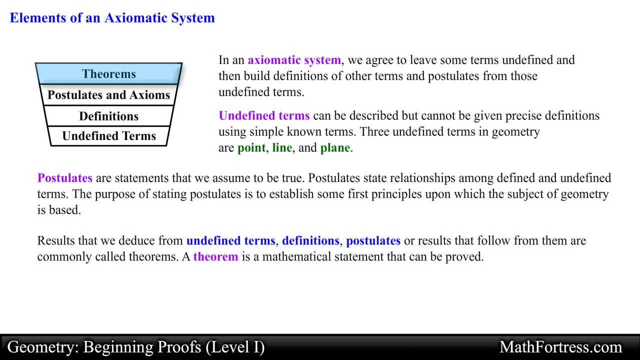 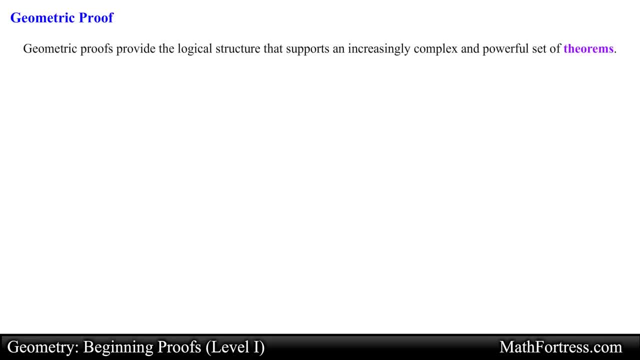 from them are commonly called theorems. A theorem is a mathematical statement that can be proved. Geometric proofs provide the logical structure that supports an increasingly complex and powerful set of theorems. In a general geometric proof, the premises are definitions, postulates, properties and 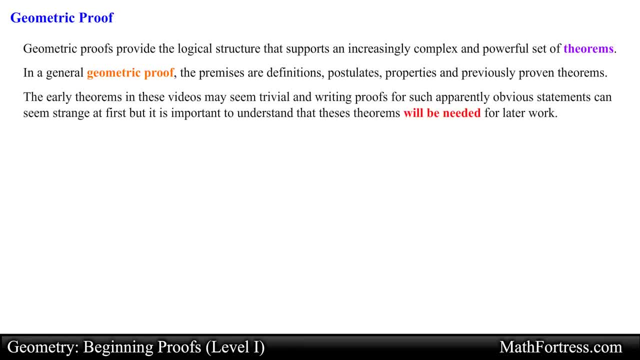 previously proven theorems. The early theorems in these videos may seem trivial, and writing proofs for such apparently obvious statements can seem strange at times. Postulates, properties and previously proven theorems. The early theorems in these videos may seem trivial and writing proofs for such apparently.